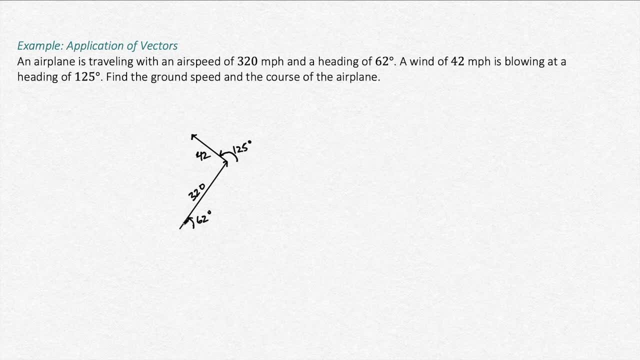 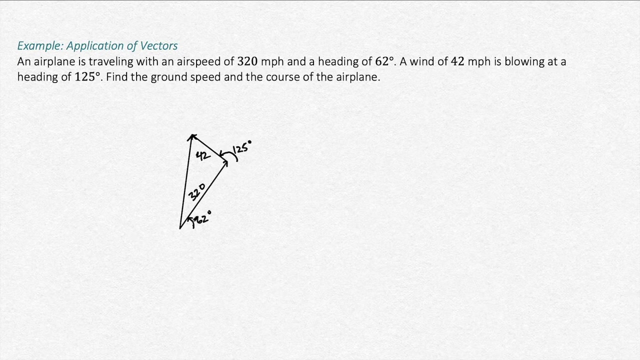 We're looking for what that oops, what that airplane ends up doing, which is this resultant right here. So that's the sum of these two vectors, And in order to find that sum, we are going to need the components of these vectors. 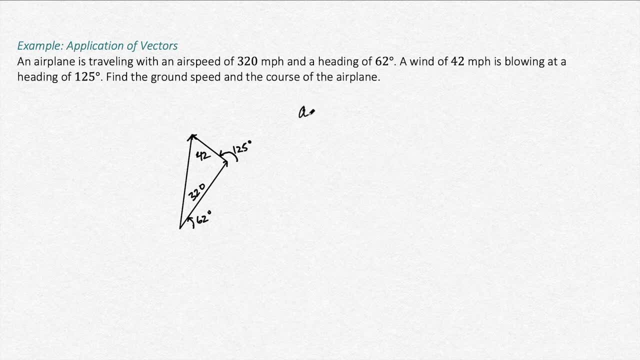 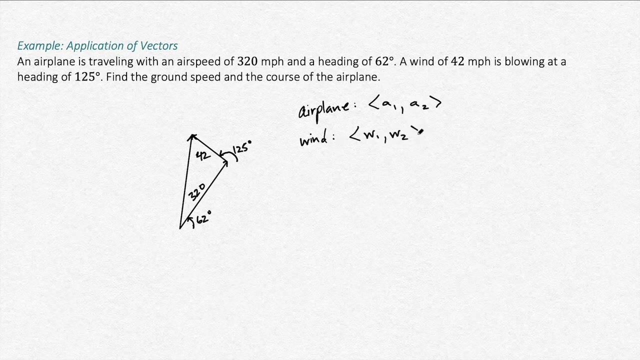 So we'll let the airplane components, the airplane, we'll let that vector be A1, A2, A for airplane, And the wind, we'll let those components be W1 and W2.. So, using what we know about components of the vector, 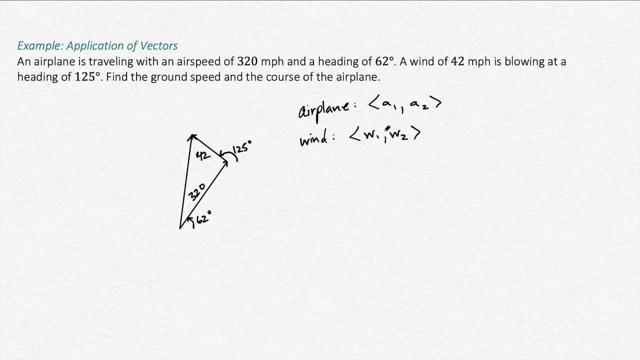 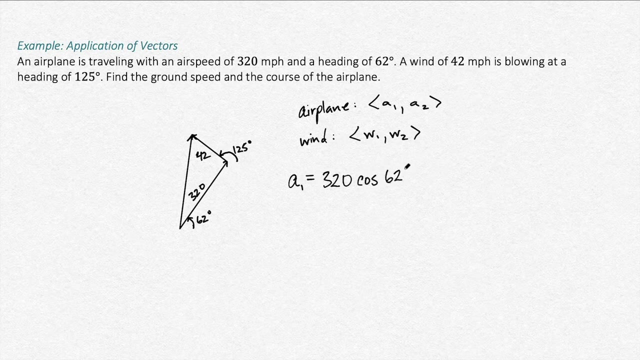 and how it relates. how they relate to the direction, the angle and the magnitude we can get each of these components. A1 is the magnitude of the airplane vector, which is 320 times the cosine of the angle: 62 degrees. 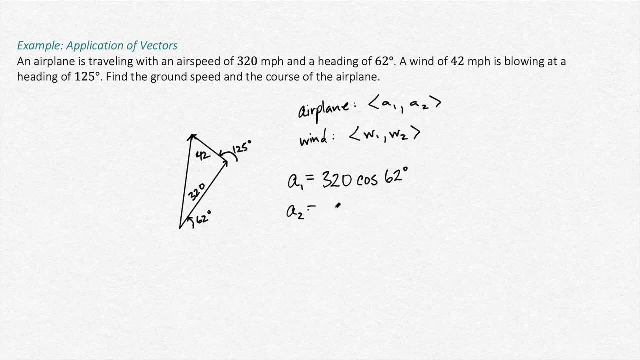 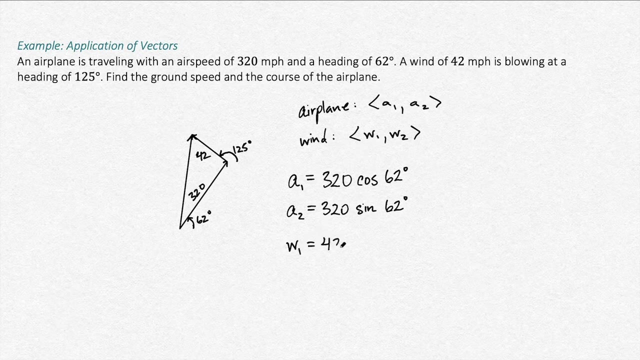 A2 is the magnitude 320, times the sine of the angle, 62 degrees. and then do the same thing for the wind. The horizontal component is the magnitude of the wind, which is 42, times the cosine of the direction angle. 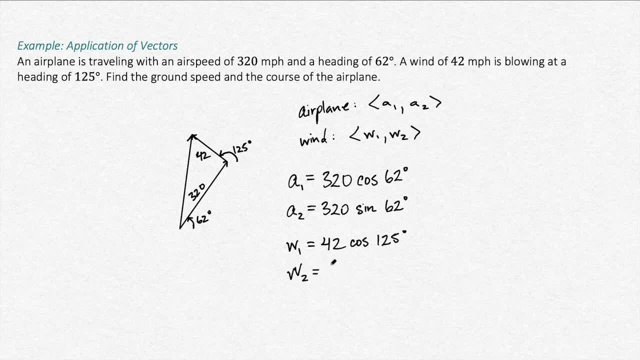 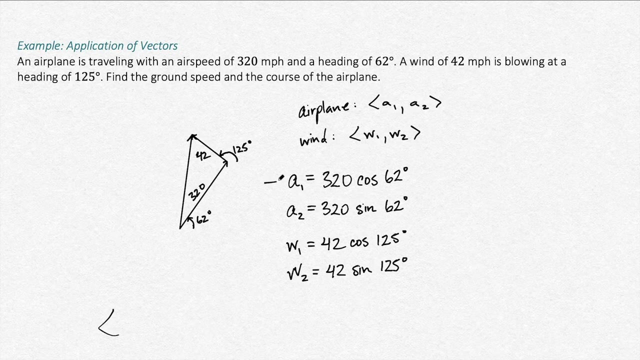 and the vertical component is the magnitude times the sine of that angle. So now we're looking for the sum of those airplane plus wind, So that's going to be A1 plus W1, these two here Go ahead and just write that. 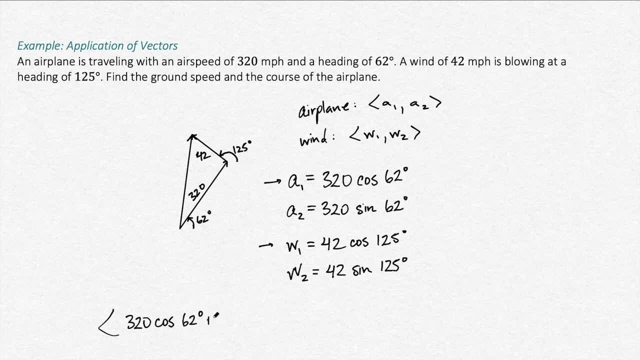 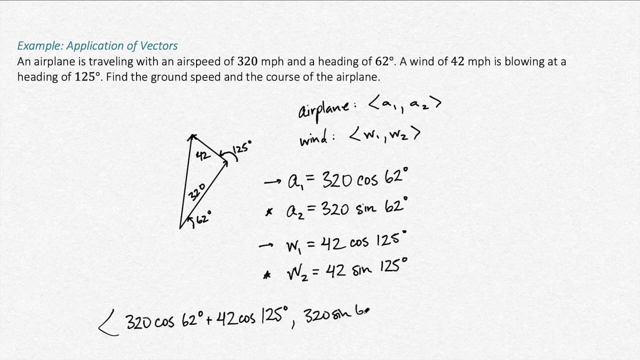 32, 320 cosine of 62 degrees plus 42 cosine of 125 degrees, And the vertical component is the A2 and W2.. Go ahead and add those together: 320 sine of 62 degrees plus 42 sine of 125 degrees. 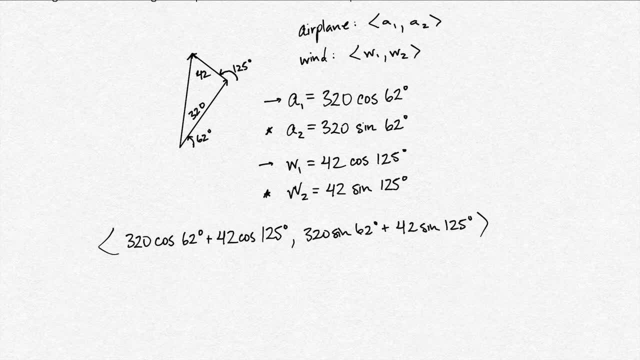 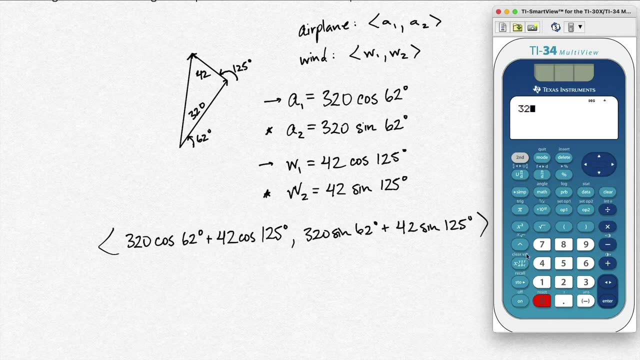 And that is what then we want to compute. I'll go ahead and plug these into our calculator, So we have 320 cosine of 62, plus 42 cosine of 125.. I'm in degree mode, so I'll go ahead and hit enter here. 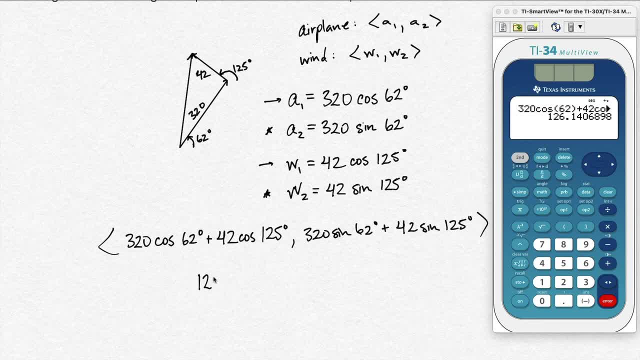 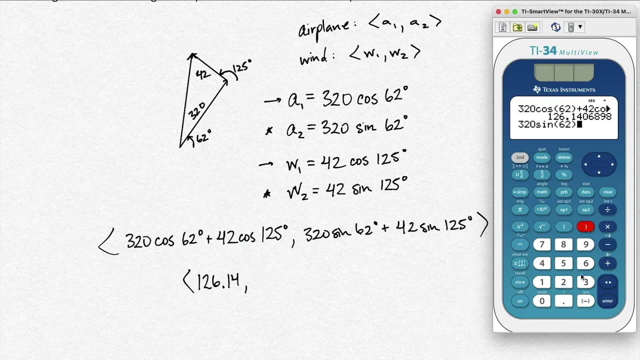 And that gives me that first component about 126.14.. Now for my second component. I have 320 sine of 62 degrees Plus 42 sine of 125 degrees, And go ahead and hit enter and we get 316.95.. 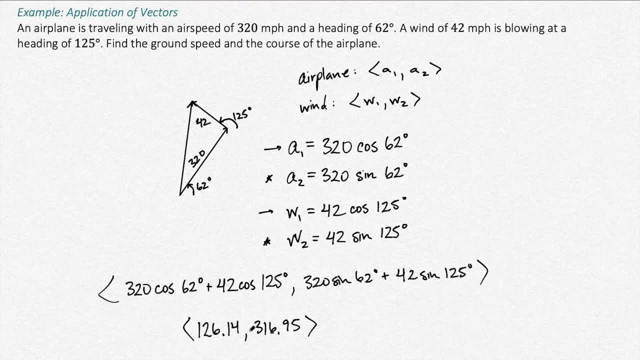 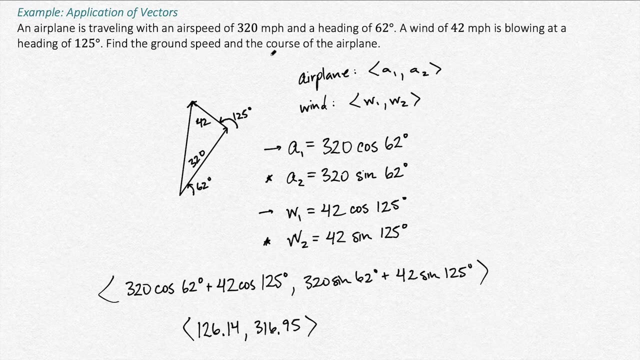 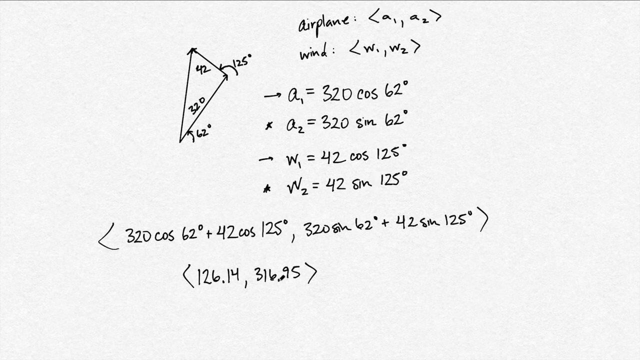 So that is the components of the vector. that is the course of the airplane After taking into account that wind. The question is: find the ground speed and the course of the airplane. Well, we have these two components, but that's not really the ground speed. 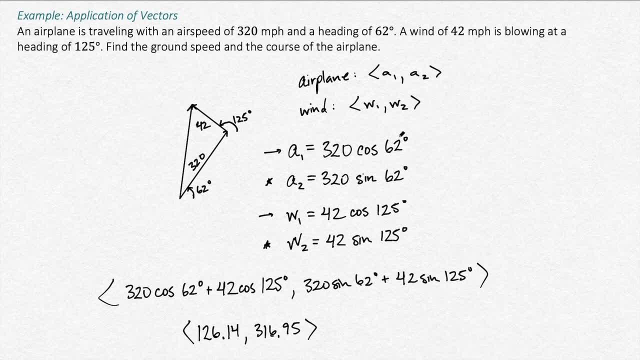 or the heading. You could make an argument that it is the course, But let's go ahead and find the heading, the angle as well. So we'll start with the drawing. just a quick little picture actually. So we've got this. 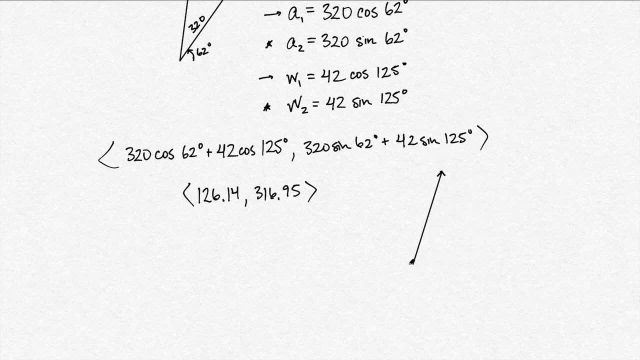 this angle, or sorry, this new vector, And we are looking for the length of it. And then, of course, this angle here, As far as the magnitude of it, we have a formula for that. We know that the the magnitude of this. 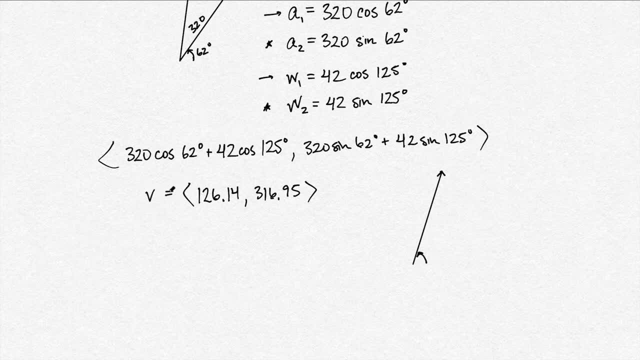 I'm going to do this. we'll call this vector v, So the magnitude of v, of course, is the square root of the sum of these two components squared, And I'm going to make sure that when I'm actually computing this, 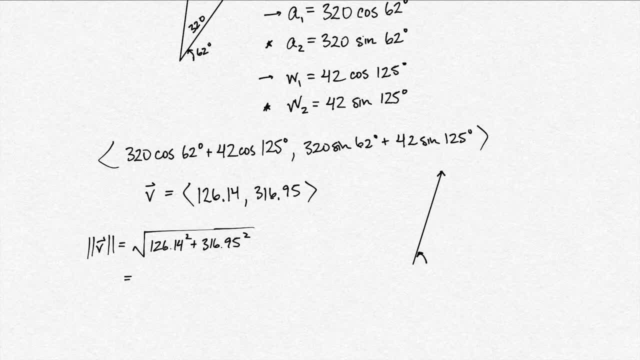 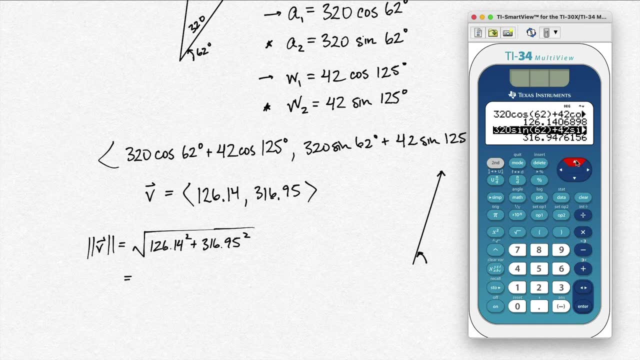 I'm using the exact forms that I got in my calculator. So back to my calculator. Those were my two numbers And I'm going to. I'm going to use those full, exact numbers. I'm going to come up and highlight, Hit, enter. 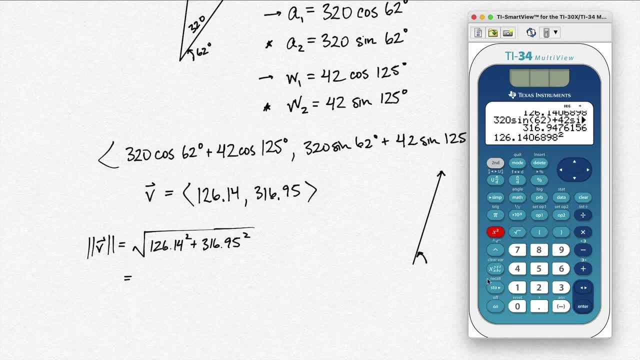 So I've got that number, I'm squaring it, And then, plus, I've got the other number, That's this one there And I'm squaring that, And I forgot to do my square root. It's okay, Hit enter. 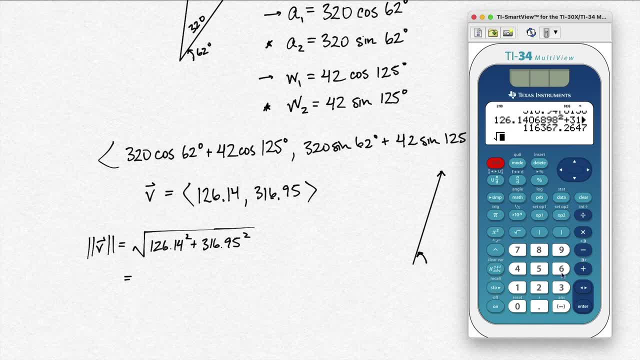 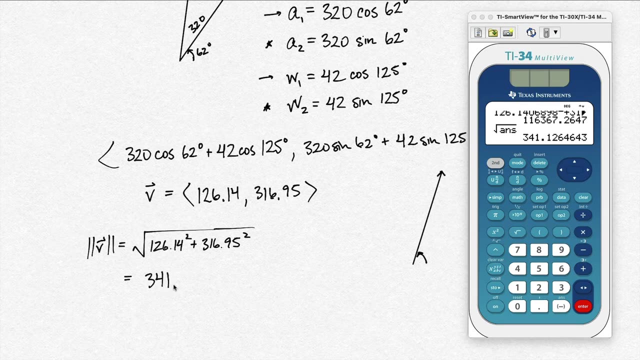 And then we'll take the square root of that answer. So there is my magnitude of this vector. This is the ground speed of the airplane, So about 341.13 miles per hour. Now we're also looking for this angle here And actually 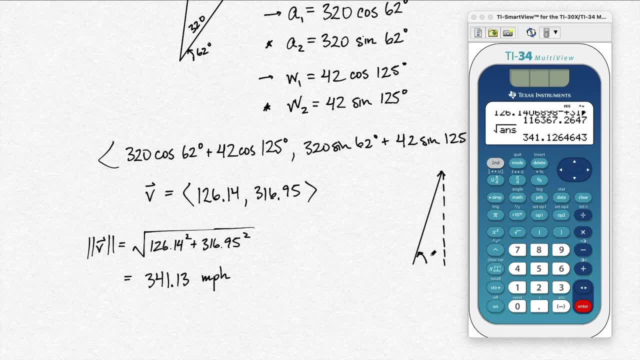 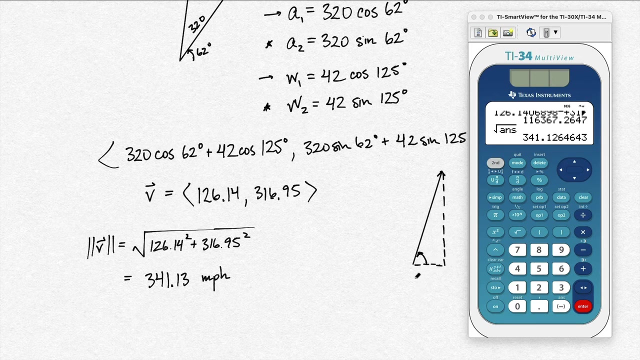 we can get that by going to this triangle, The angle, I should say the acute angle, that the vector makes with the axis, the x-axis I can think of as an inverse tangent, where I've got my vertical component here, my horizontal component. 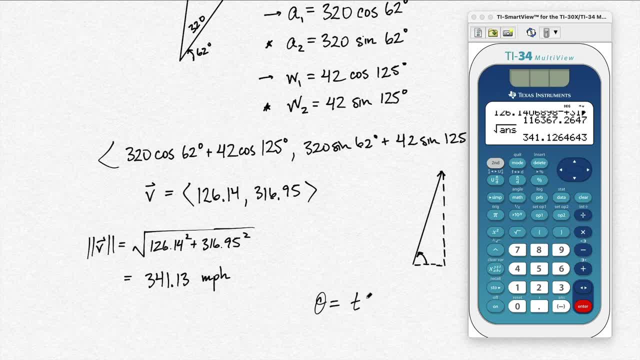 To get this angle, theta, we're going to take the inverse tangent of the vertical component divided by the horizontal component, right opposite over adjacent, So that's going to be the 316.95 over the 126.14.. Now this is, of course, 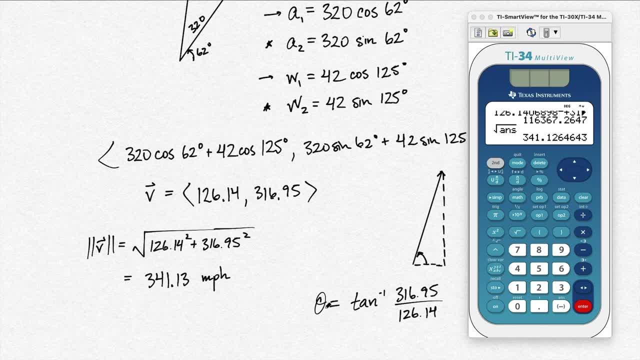 just the acute angle, that, the angle that the vector makes with the x-axis. You do have to check the quadrant in order to actually find the heading of the vector, the actual angle. Let's go ahead and do this. here We've got the inverse tangent. 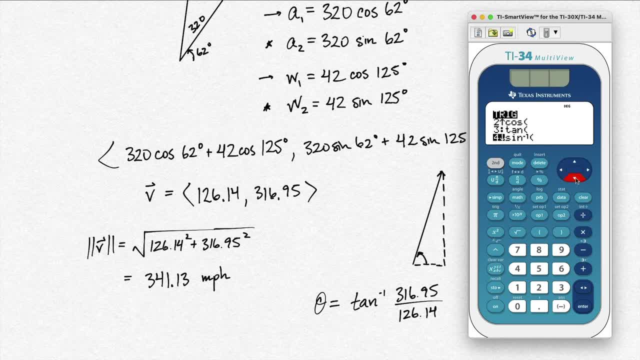 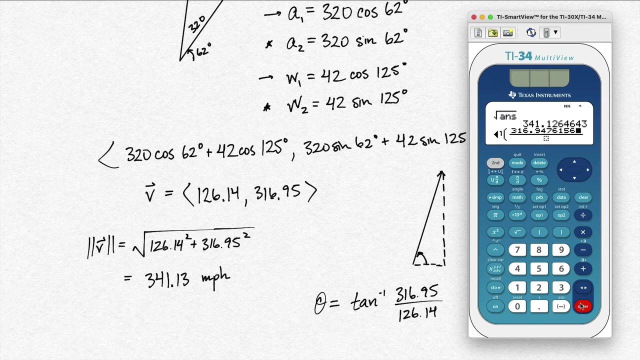 So I'm going to go into my trig and go down to my inverse tangent of a fraction And that fraction is: let's see if I can pop those numbers in. I had my 316 right there And then divided by. unfortunately I didn't. 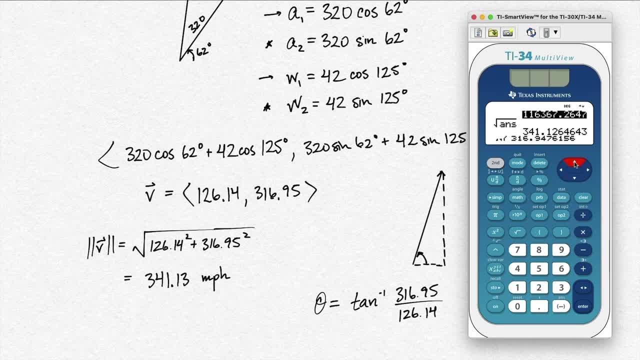 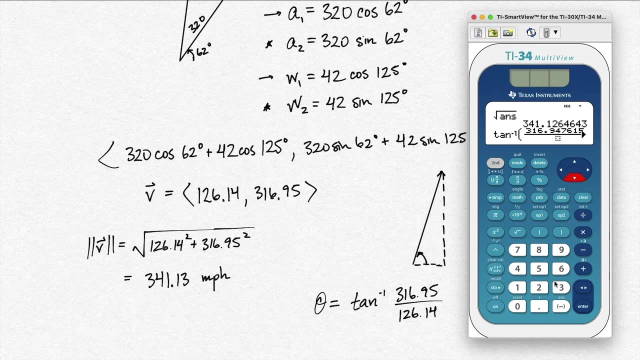 I can't copy, It's not going to. I don't think it's going to quite work. I'm just going to go and copy it down. So 126.1406898.. 06898.. All right, And then hit enter. 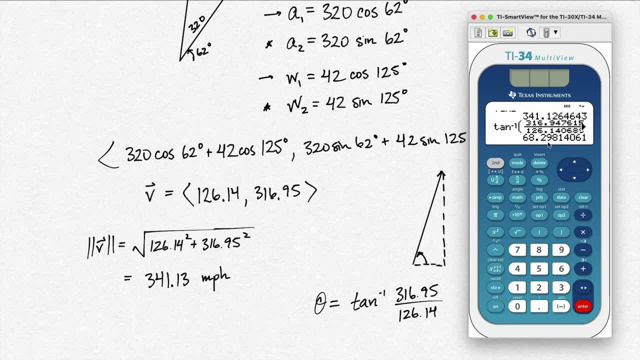 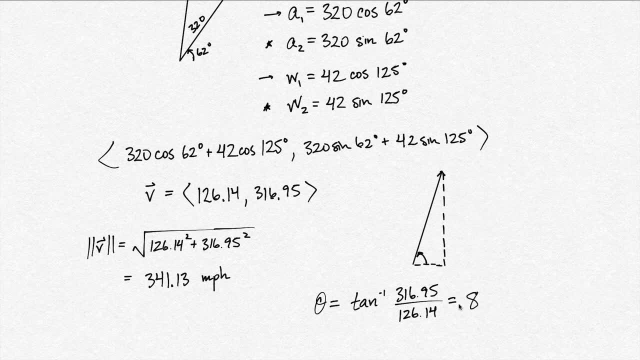 And that gives us our acute angle. I'll round that to 68.3.. So 68.3 degrees. Now this is the acute angle that my vector makes with the x-axis, Because both my horizontal and vertical components of the vector are positive. 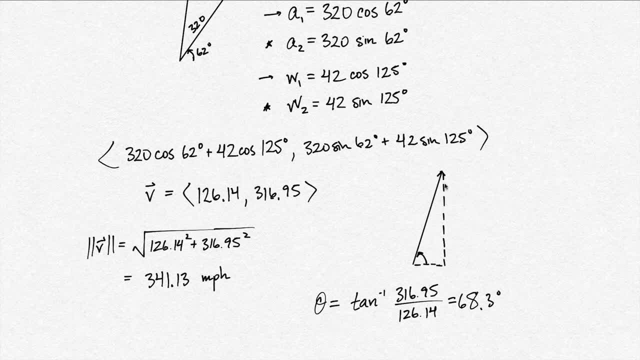 I know that my vector is in the first quadrant, And so this is the correct angle. If the vector had been, say, in the second quadrant, like somewhere over here, I'd be looking for this full angle, but the inverse tangent would have given me this angle. 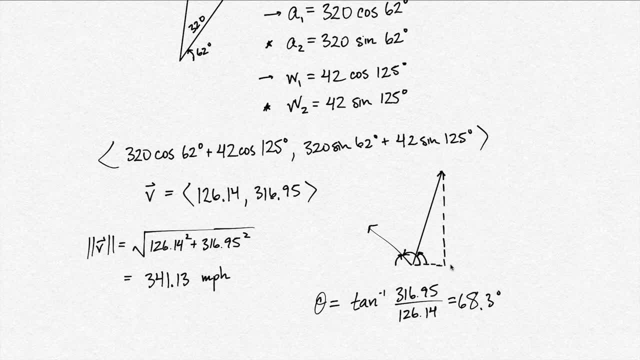 And so I would have gotten my heading with doing 180 minus the angle that I got. So you just have to think through what the angle is that you actually are trying to find and what the inverse tangent actually gives you, And so that's just. what this X-axis does. And then here we go. See, It's obviously in the correct angle. I'm going to try and get that y axis into this one, and then we'll have our first Ellipse in here, And that's our X-axis. So now this x-axis.